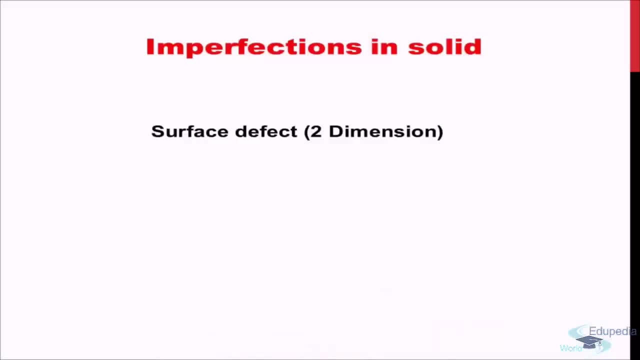 dimensional defects. Two dimensional defect is also known as surface defect, right, Because a surface is basically a two dimension. So what are the possible type of surface defects? It can be an external surface. The ending of the specimen- right. So any specimen will end somewhere, abruptly. So. 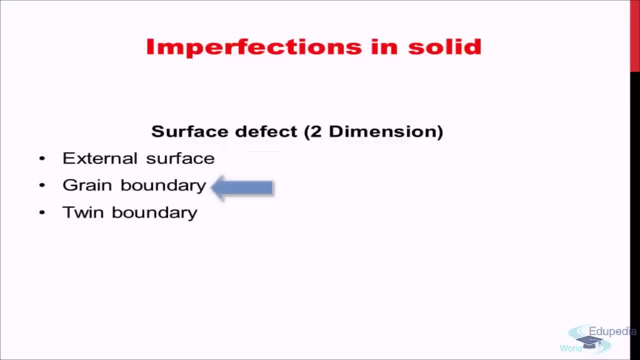 it has an external surface. Then there will be grain boundaries. I have already discussed about grain boundary in previous lectures, but I will go and discuss about it in further details today. And then we have something known as twin boundary. It's a special case. 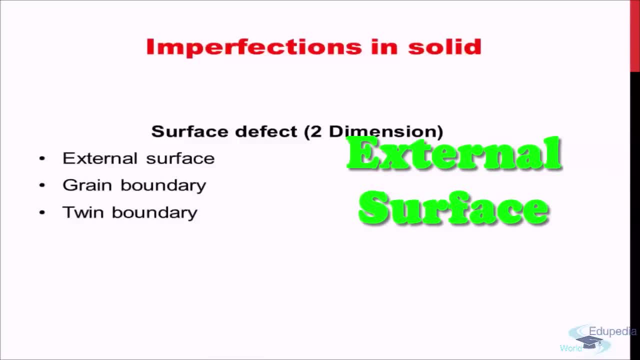 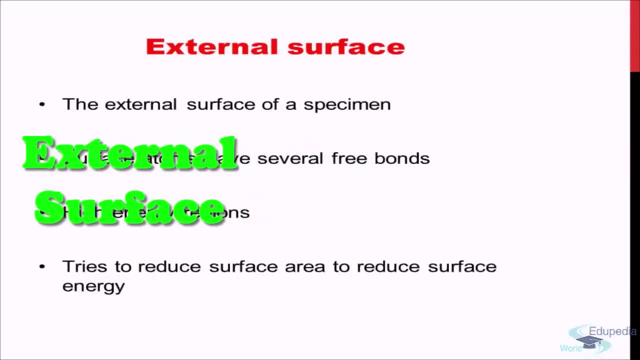 of grain boundary. So let's start our discussion with external surface. So, as the name suggests and as I said, external surface is basically the ending of the specimen right, The external surface of the specimen. So what happens is that normally, if there, 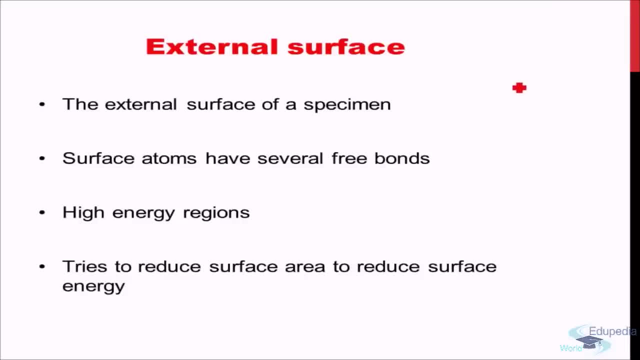 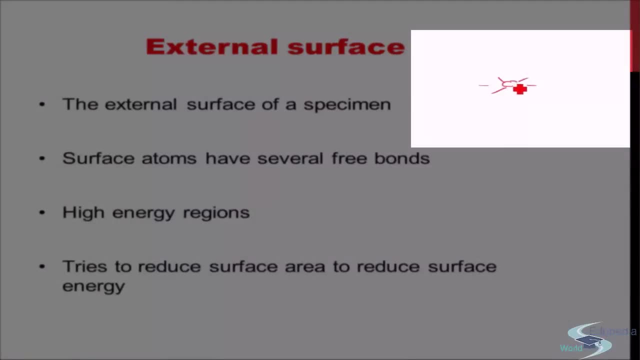 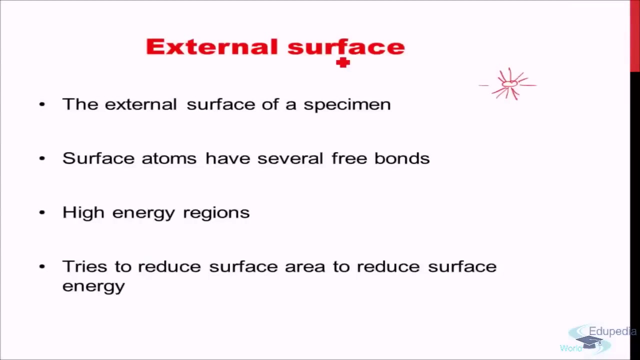 is an atom, it will have a coordination number. Let's say we have a FCC kind of atom, then it will have a 12 coordination number, which means there will be 12 bonds attached to it, right? So in this plane, 3 top and 3 bottom, That will make the 12 bonds for this atom. and when? 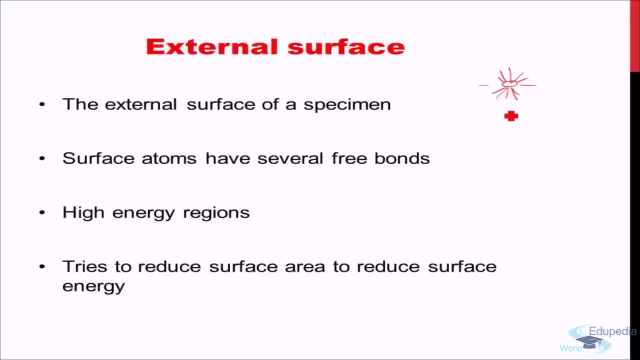 all the 12 bonds are present. it is surrounded by all the possible atoms in all the possible directions. right, But what happens at the surface? When we have surface? an atom at the surface will have less than the maximum number of possible bonds. 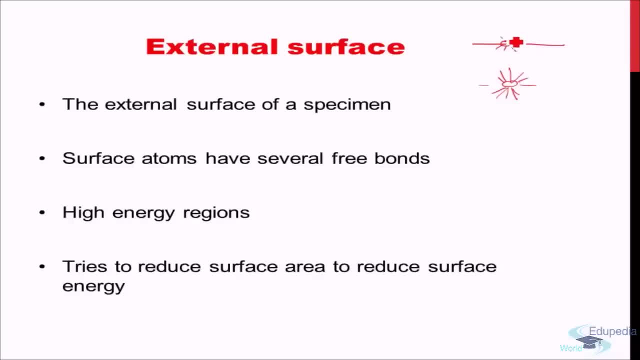 Thereby there will be loosely hanging bonds, There will be free bonds, and free bonds means higher energy, because bond formation leads to release of energy, thereby lowering of energy. That's why, basically, bonds are formed: in order to lower the energy. But the external surface. 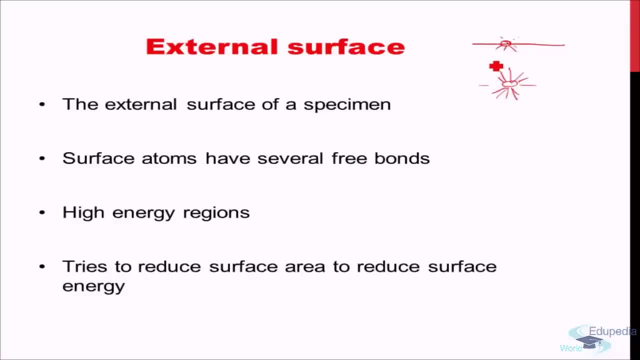 atoms will have free bonds, Thereby they will have higher energy. Therefore, as I have written here, external surfaces are regions of high energy Because they have free bonds And the ideal case- the material would try to minimize the surface, external surface area. Therefore, during solidification, what will happen is 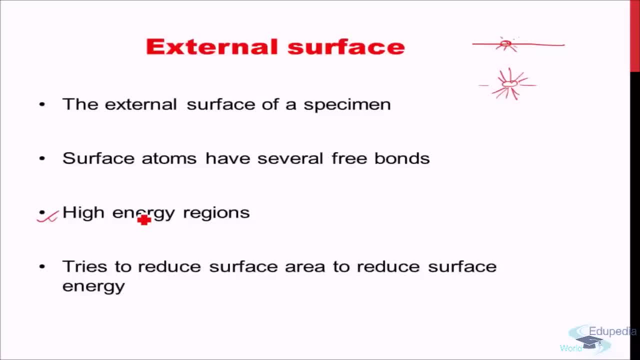 they will try to solidify in a spherical manner, right, But once the solid is there, it is intact and there cannot be any possible changes in the surface area. okay, So this gives you an idea about external surface. And why is this called a defect? This is a defect because, basically, the atoms does not. 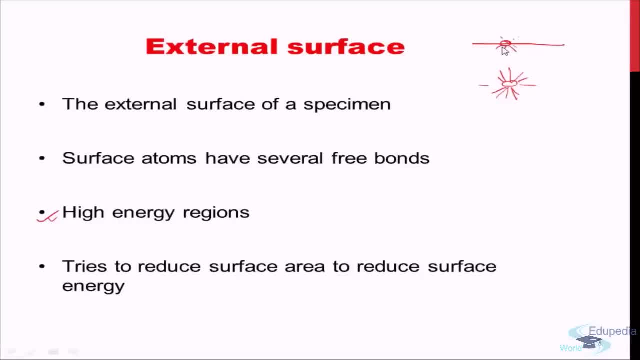 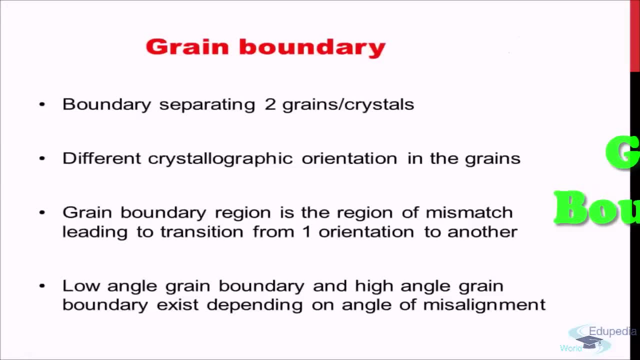 have the type of bonding which it is supposed to be if it were in the bulk right Now let's jump into the more important type of two-dimensional defect, that is, the grain boundary. If you remember correctly, I have discussed that any material is composed any 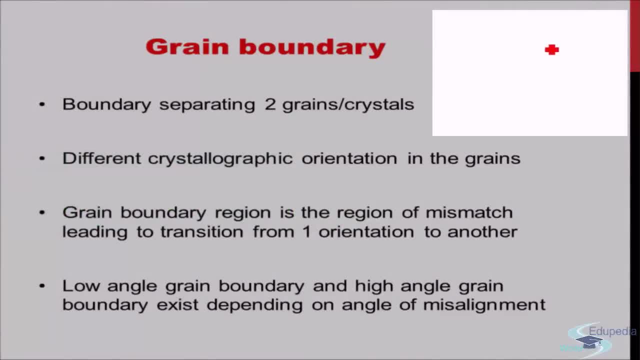 crystalline material is composed of many grains. right, There will be different grains like this And each grain will have a particular crystallographic orientation. So something like this And the change in crystallographic orientation is basically the boundary where the change of crystallographic orientation takes place. 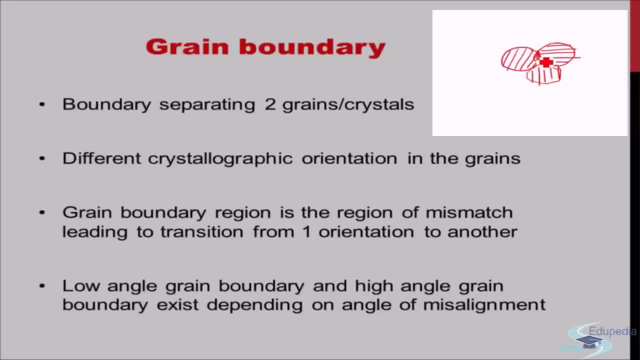 is known as the grain boundary. So between this and this grain there is a change in crystallographic orientation over here and a change in crystallographic orientation over here and here. So these are the grain boundaries. Grain boundaries are basically regions which 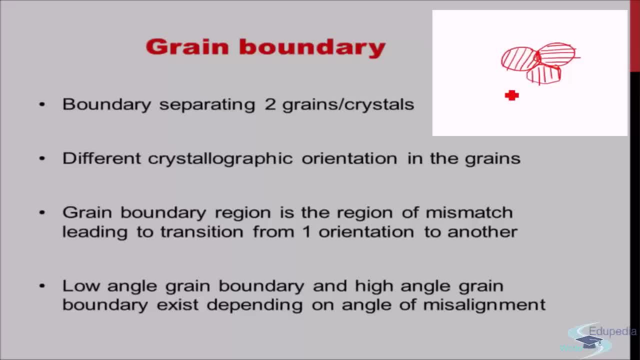 are separating two different grains or crystals. okay, And, as I already discussed, different crystallographic orientation is present in different grains. Grain boundary region is basically, then, what it is: It is the region of mismatch, leading to transition from one orientation to a different orientation. 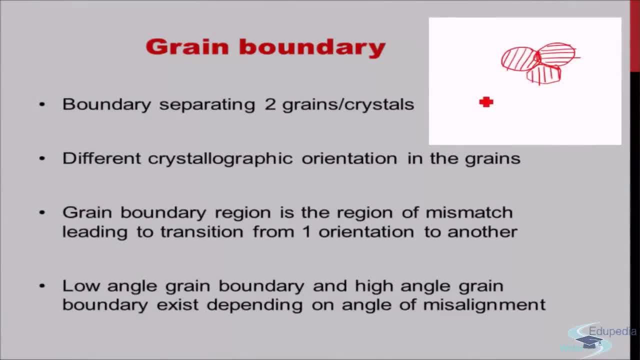 Okay, in terms of atomic arrangement, if you think. suppose in one grain we have atoms arranged, perfectly, arranged like this right, Perfect arrangement of atoms like this, But in the adjoining grain the atom arrangement changes. So what we get is that in the adjacent 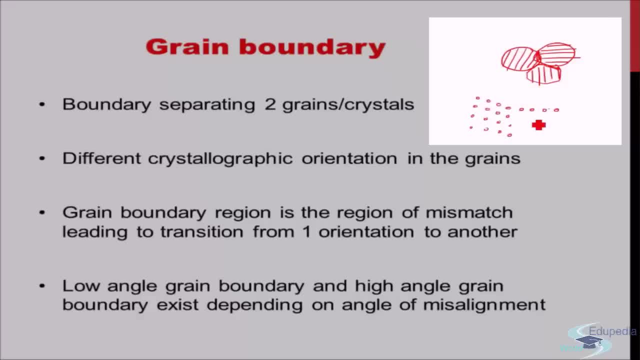 grain we have atoms arranged in a different way, right? If you think about it, suppose in one grain we have atoms arranged in a different way. If you think about it, suppose atom arrangement changes. So like this, right? So what is happening Here? the orientation is: 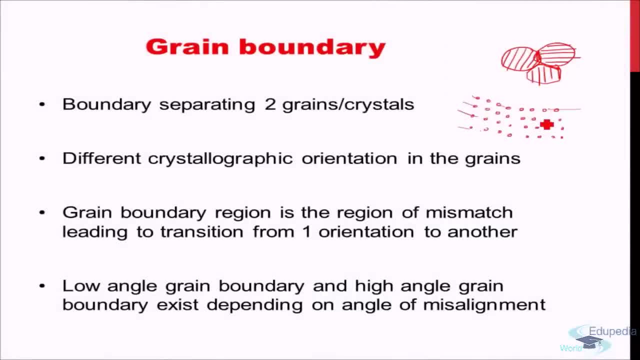 in this fashion, whereas here the orientation changes to this fashion and a clear demarcation over here takes place. where the atoms are not exactly located where they should be, either from the atoms of this grains perspective or from the atoms of this grains perspective, There is 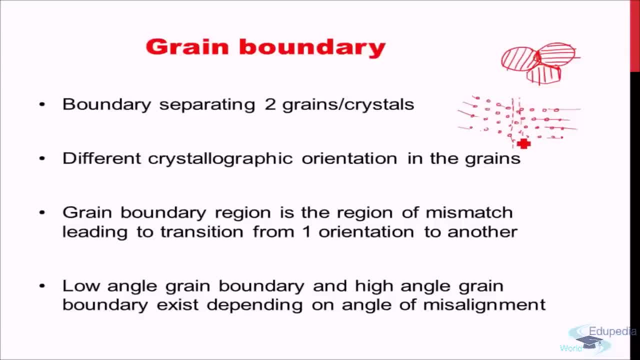 internal region where the atoms are randomly placed. They are not perfectly aligned with the grains. So this region is basically our grain boundary region. We can have two types of grain boundary: We can have low angle grain boundary or we can have high angle grain boundary and that 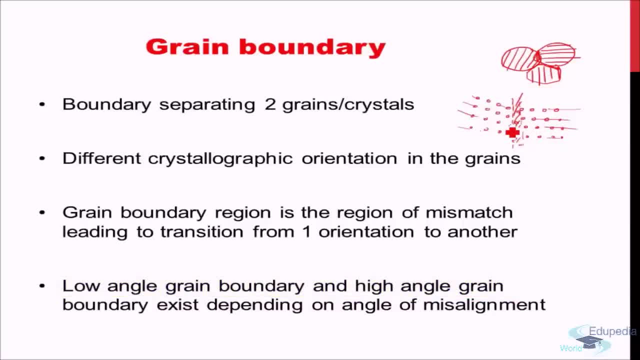 will depend on the degree of misalignment. If the grains are almost similarly oriented but there is, let's say, a misorientation of around 4 degrees, 5 degrees, then this falls under the low angle grain boundary type. But if one grain is like this and the other grain is, 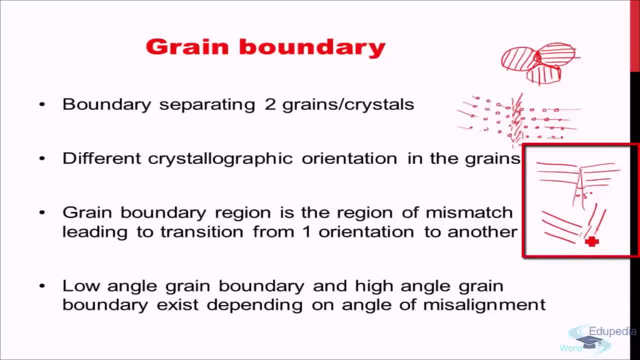 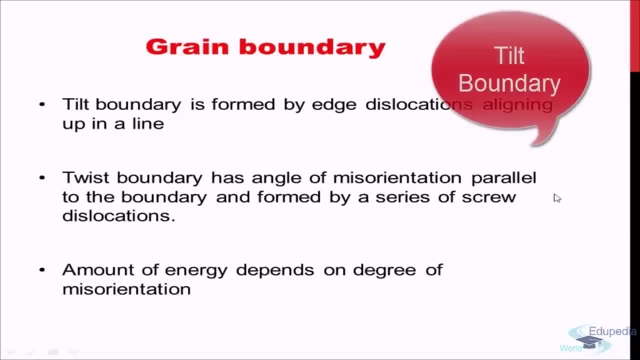 like this, then what is happening? We'll have a very, very high angle of misorientation. This theta is very high, and then this is a high angle grain boundary region. Okay, now grain boundaries can come into variety. One is the tilt boundary and the other is the twist boundary. 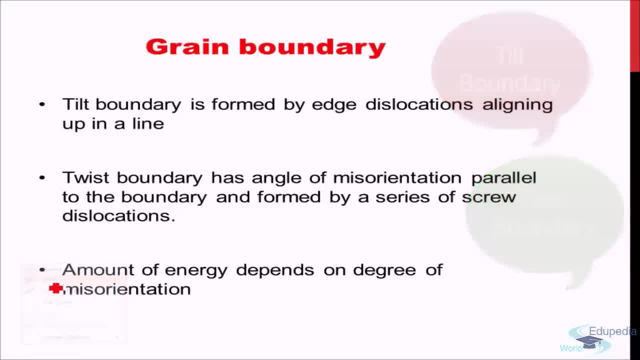 What is tilt and what is twist boundary. Tilt- boundary is basically formed by edge dislocation, lining up. So there will be several edge dislocation like this: Okay, and atoms are arranged like perfectly over here and perfectly over here, But the misorientation is taken care of by 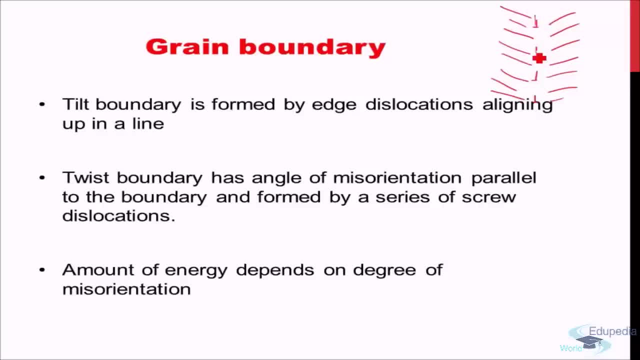 a series of edge dislocations In the grain boundary region, Whereas a twist boundary is something where, instead of edge dislocation, the misorientation is taken care of by screw dislocations. And how does the misorientation takes place Here? the atoms in the tilt boundary atoms are 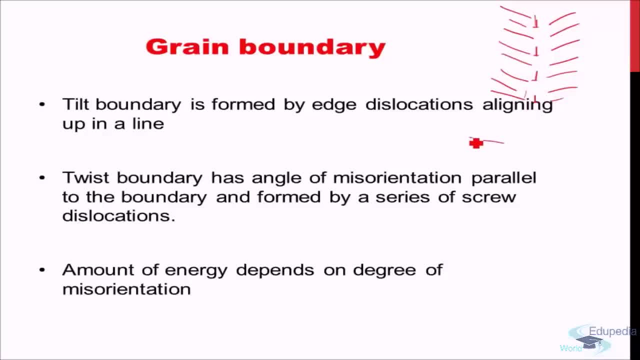 like this and this In the twist boundary. basically, you can imagine this as atoms arranged perfectly here and there is another cube, Okay, Another cube like this, where again the atoms are perfectly arranged, But this cube and this cube are inclined at an angle to each other, Right? So basically there is a twisting. 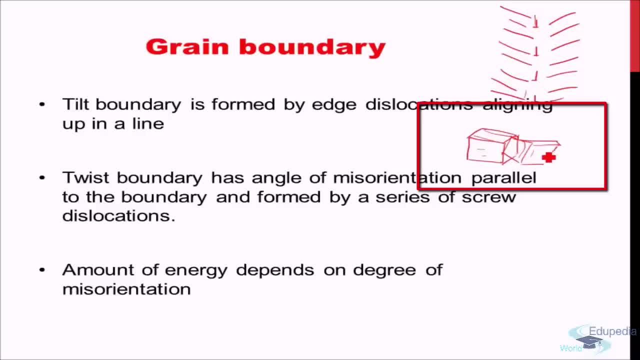 of the atoms. The atoms in this arrangement is twisted with respect to the atoms in this arrangement. So basically, you just provide a twist for all the atoms and this can be taken care of by a series of screw dislocations. Okay, So this are the two types of Grain Boundaries that can be there And obviously the amount. 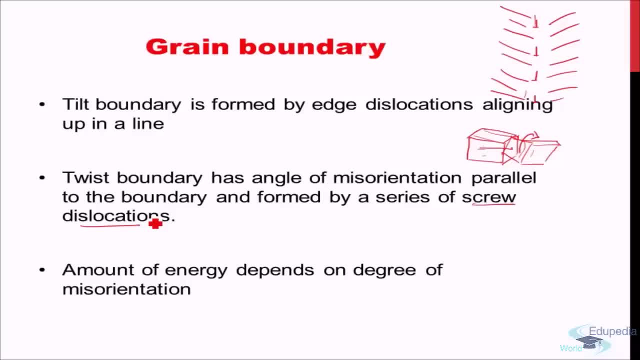 of energy that is present in a grain boundary depends on the amount of disorientation, the degree of disorientation. Larger the degree of disorientation, more will be the number of dislocations to take care of the misorientation and more will be the amount of energy in the. 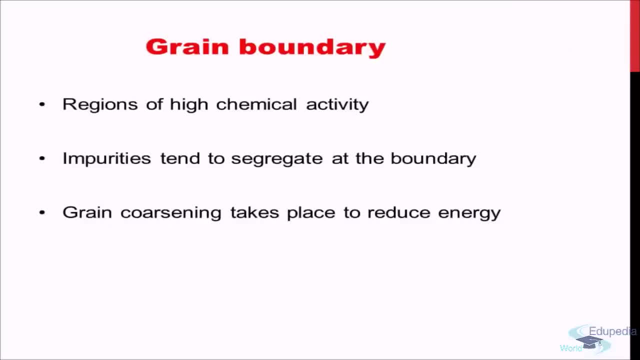 Grain Boundary. Fine. Now, as I said that grain boundaries are regions of higher energy Because there are defects present, un-uniformity. Therefore, since it is a region of higher energy, it is also a region of higher activity, higher chemical activity. Why so? Because by high chemical activity, the grain 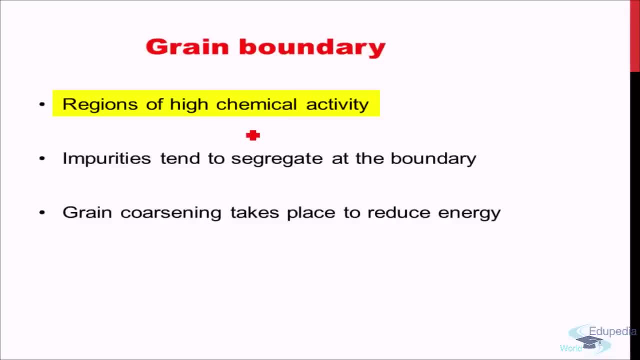 boundary region tries to reduce its energy. It tries to pull down the energy and attain a more stable state. For the same reason, impurities tend to segregate at the boundary. If there are impurities present in the material, they will try. if like suppose these are different. 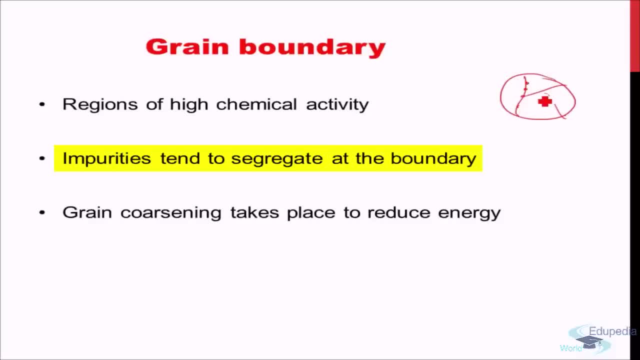 grains, then the impurities will come and settle at the grain boundaries, Because these are already regions of high energy and the impurities, if present in the bulk, will lead to higher energy. So they rather sit at already high energy region and thereby reduce the 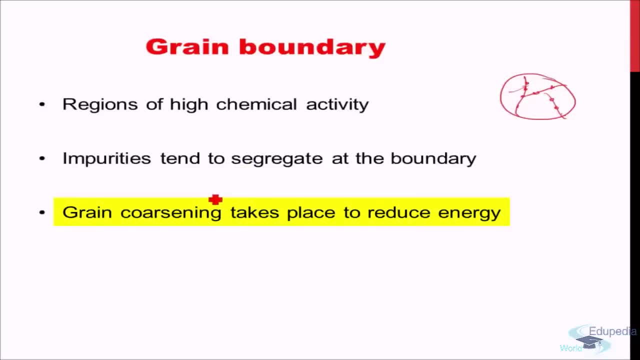 effective energy of the whole system. And finally, as we have seen, that grain boundary region is a region of higher energy. So if there are impurities present in the grain, boundary region is a region of higher energy. Therefore, if the total effective 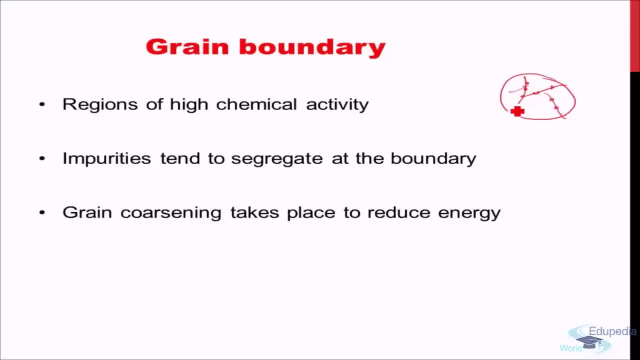 surface area of the grain boundary is less, then the effective energy of the system will reduce. And how can we reduce the total surface area? We can reduce the total surface area if, instead of many small grains, we have less number of coarser grains. right So the effective 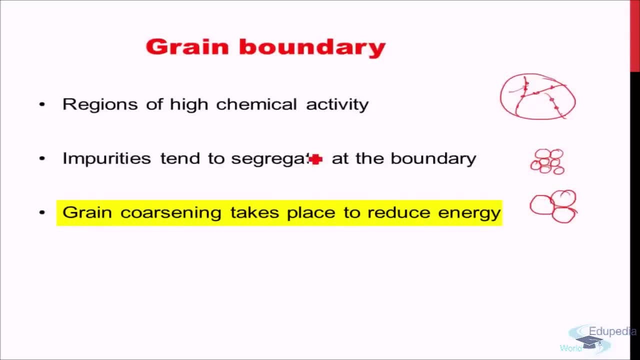 surface area will be reduced by coarsening of the grain, which is known as grain coarsening, And this is one of the reasons why we have to reduce the effective energy of the system, And this is one of the methods which is used to reduce the surface energy of the, due to. 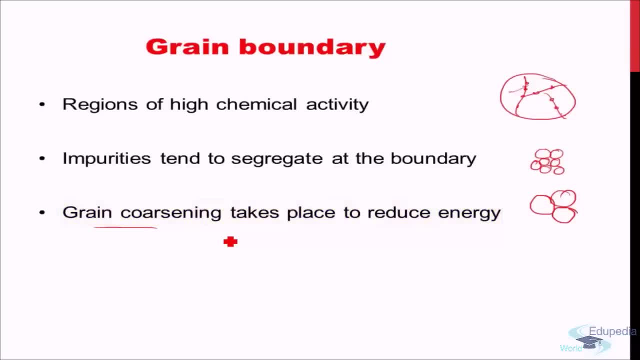 the grain boundaries. Okay, So just to sum up the idea that grain boundaries are regions of mismatch of crystallographic orientation And they are a series of either edge dislocation in tilt grain boundary or screw dislocation in twist grain boundary. So this is one of 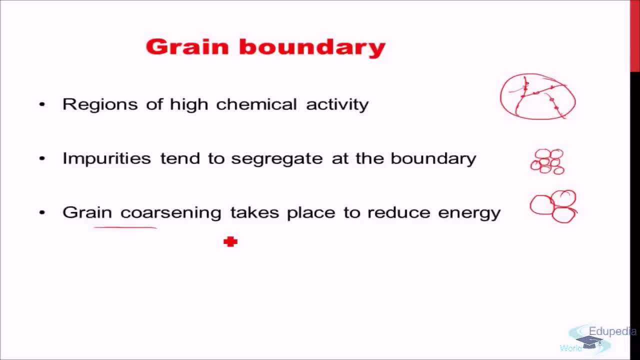 the reasons why we have to reduce the amount of coarseness of the grain boundary or screw dislocation in twist grain boundary. Okay, With this background, let us see the 3rd type of 2-dimensional defect. The 3rd type of 2-dimensional defect is a special kind of. 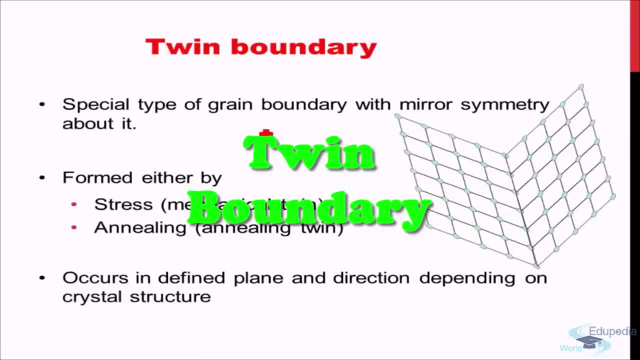 grain boundary, It is known as twin boundary. We have seen in the case of grain boundary there is a mis-orientation right. But in the case of cross burst 수 it will aim to not be 하겠습니다 with the捩 boundary And it will이다 to the solid correct트 of gas. 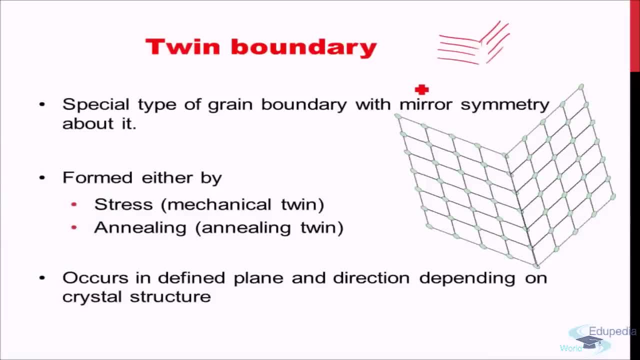 is션 in twist. Bio Variant 2auenz shell ml is spoilage. хороший strain wellbeing too. of the�� How or how does mix orientation work? for the 2 Guru rain boundary, twin boundary, there is a symmetry in the misorientation That is this image represents. 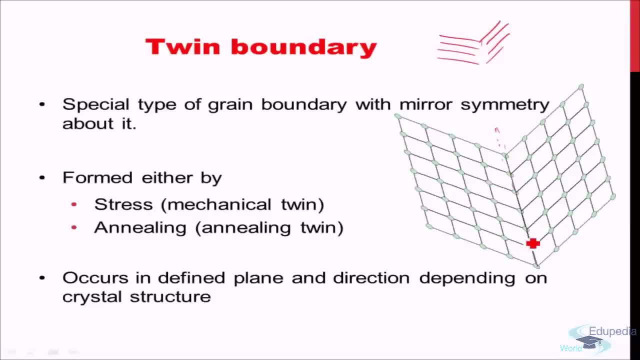 a twin boundary. What is happening is that this is the twin boundary and for every atom in this grain there is an equivalent atom, a mirror image, if you would like to say So. they exist in pairs. For every atom here, there is another atom in the other grain, right? So a special. 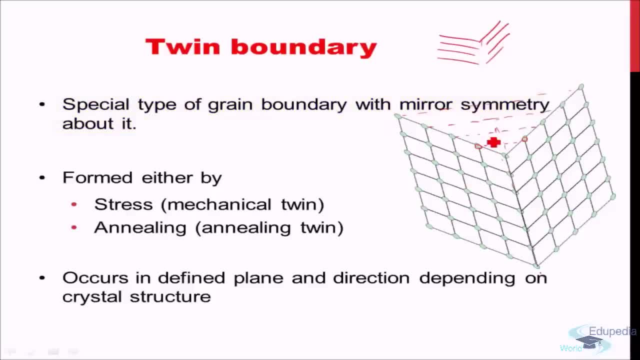 type of grain boundary, with mirror symmetry about the twin boundary, rather. Now, how does twin boundaries form? There are two types of twin boundaries. Twin boundaries can either be formed due to stress, which is known as mechanical twin, or it can be formed during annealing treatments. 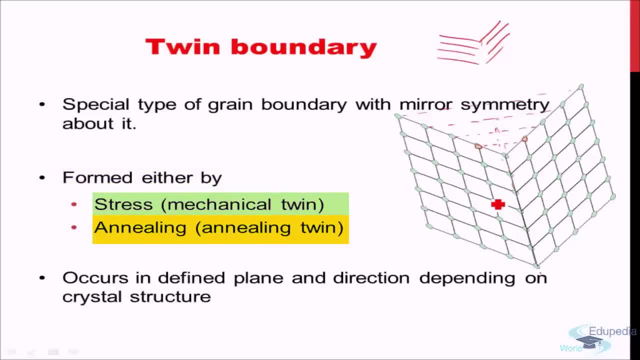 which is known as annealing twin. Okay, So these are the two types of twin boundary. They are having the same properties, but just their formation. reason of their formation is different. And twin boundaries occurs in certain defined planes and directions. And what defines the plane and direction? on? 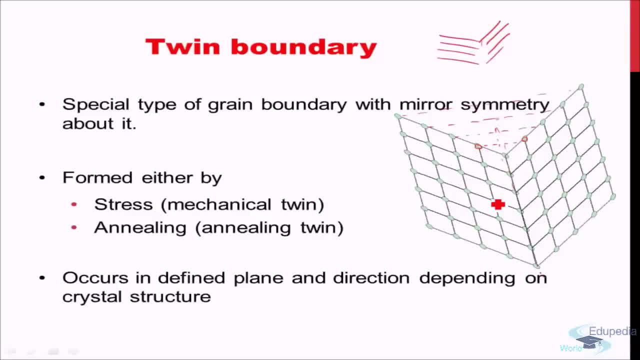 which the twin boundary will exist. It depends on what crystal structure we are discussing about. We are not going to go into the details about twin boundary. I just wanted to introduce you to the idea that some symmetry can even be present in the terms of twin boundary. 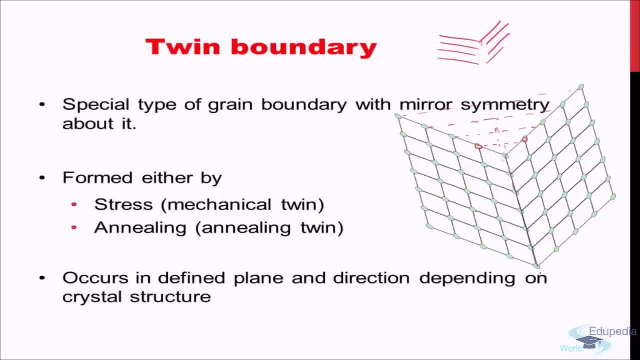 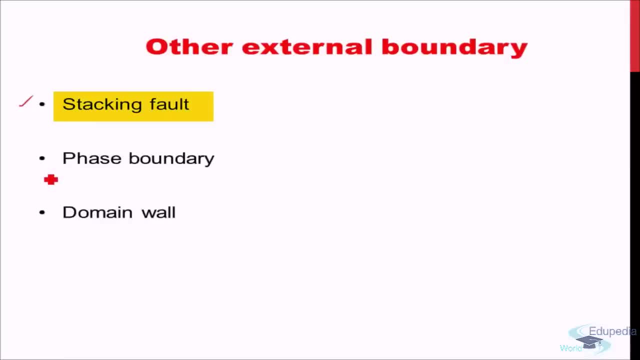 Now let us see some other two dimensional defects that can be present, Something that is known as a stacking fault. Then we have phase boundary, Then we have what is known as domain wall. Let me briefly explain you Stacking fault. I have said that ABC. ABC arrangement is present in FCC crystal right. 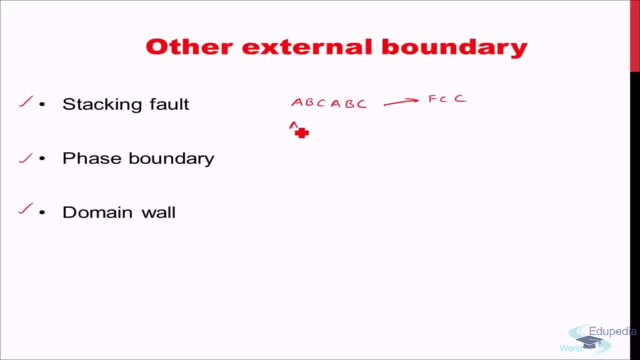 Suppose it so happens that ABC, AB, ABC and further it continues ABC, ABC. So here, effectively, what is happening is there is a fault in the stacking sequence right, The C layer is absent here. So this type of defect, this type of defect due to a change in the stacking sequence is 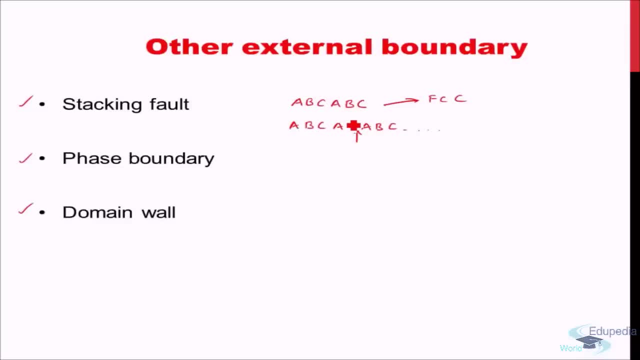 known as a stacking fault. okay, What is a phase boundary In grain boundaries? what happened is that there were different grains of the same material, of the same phase, But it can so happen that the two grains surrounding grains belong to the same phase. 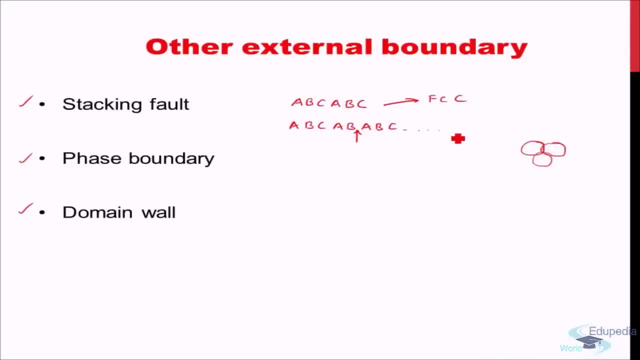 So this is a phase boundary, So this is a different phase. right, One can be ferrite and the other can be cementite. These are in. we will discuss about ferrite and cementite in iron while discussing about steel. 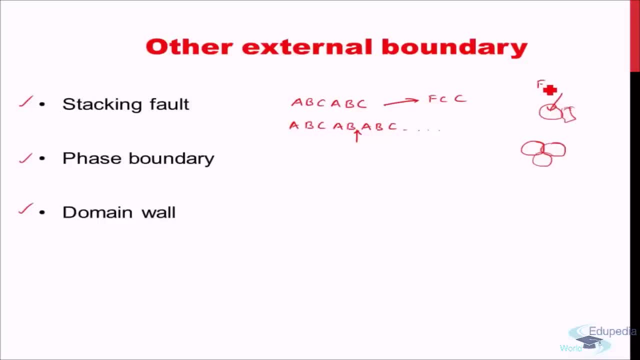 But for the time being, let me say that ferrite is one phase, cementite is another phase. Ferrite is basically alpha iron And cementite is alpha iron. Okay, So if there are two different phases present, then the region boundary separating them will. 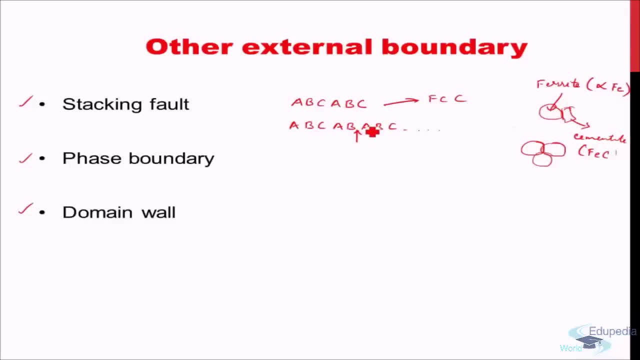 be known as phase boundary. Fine, Now, what is a domain wall? A material can be magnetic, right? So let's assume that we have a magnetic material and there will be different regions in the material Which will have magnetic Magnetic Yes. 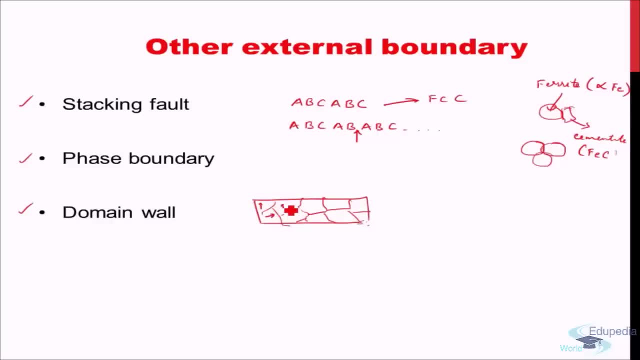 orientation in different directions. effective magnetic orientations in different direction, right. so the regions, the boundary separating these different orientations are known as the domain walls. these are different domains of different magnetic domains, so the boundary separating them are known as domain walls. so these are the different kinds of two-dimensional defect that can. 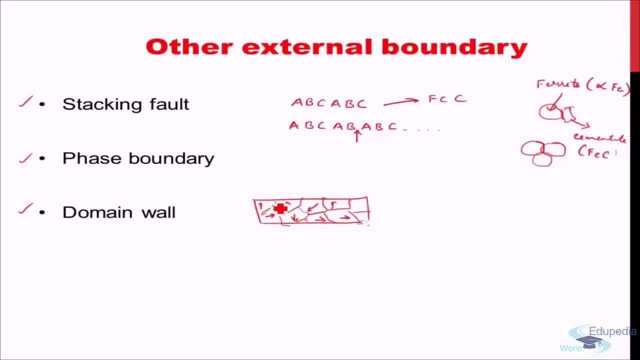 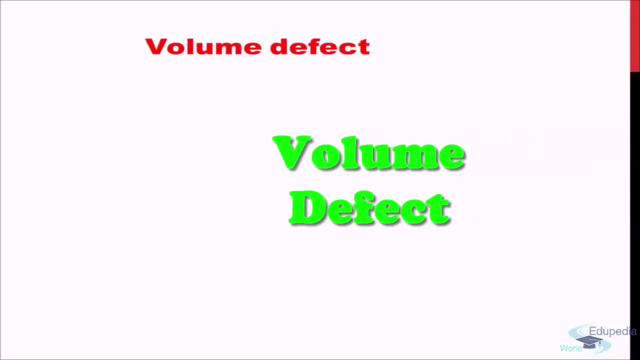 be present. now let us see briefly what are some of the three-dimensional effect that can be present in a material. three-dimensional effect are also known as volume defect, because a volume is basically three dimensions. so what can be different kind of volume defects? one can be poor, there can be porosity in the 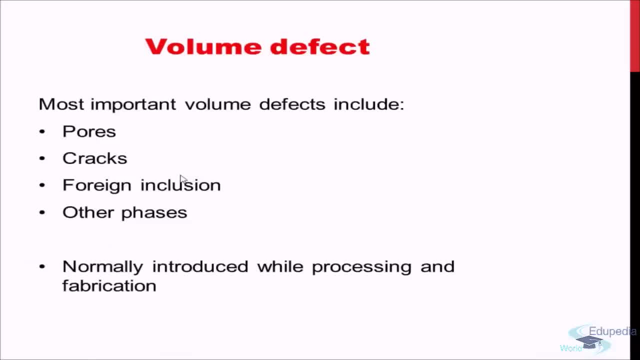 material. then there can be cracks, right, there can be cracks through the material which are not supposed to be there, but it is there. then there can be presence of completely different material, different material, as in they are known as foreign inclusions. so we have something like this with different grains of the same material. 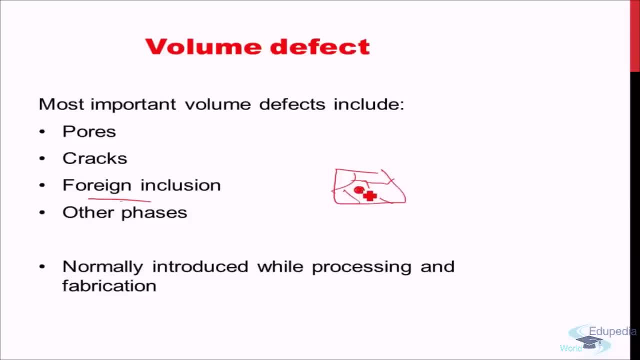 but then we have some inclusion here. so this is a three-dimensional inclusion. therefore it is a volume defect and there can be other phases present. it should not be there right at. what are the causes of volume defect? volume defects mainly occur during the processing and fabrication stage itself. 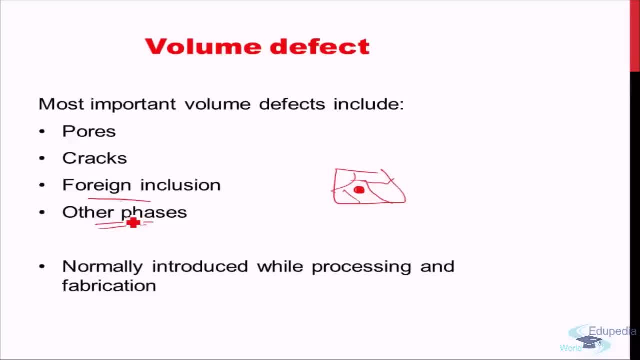 so once it is introduced in the material, it stays in the material. also, problems like cracks can occur due to usage, usage. continuous usage can lead to crack formation. So this kind of brings you to the conclusion of the lecture, series of lectures introducing you into the concept of imperfections in solid.